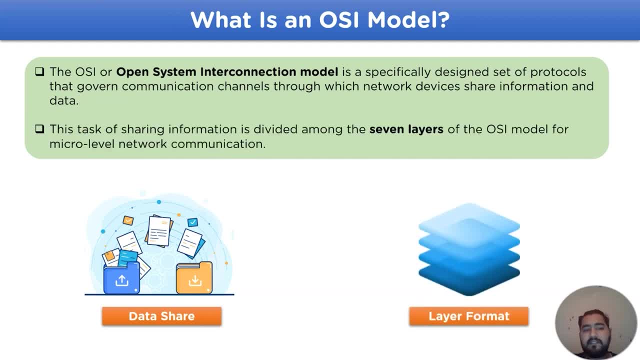 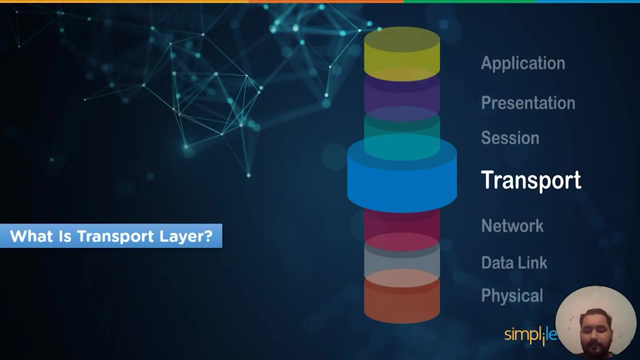 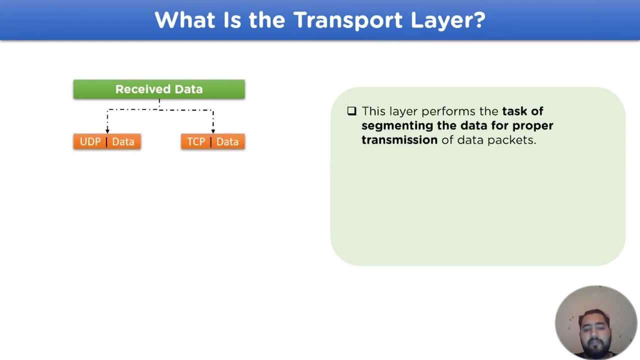 share input and data. This task of sharing information is divided among seven layers of the OSI model for micro level network communication. Now let's move on to the core topic for this session, that is, what is transport layer? The transport layer is responsible for overseeing the data being transmitted. 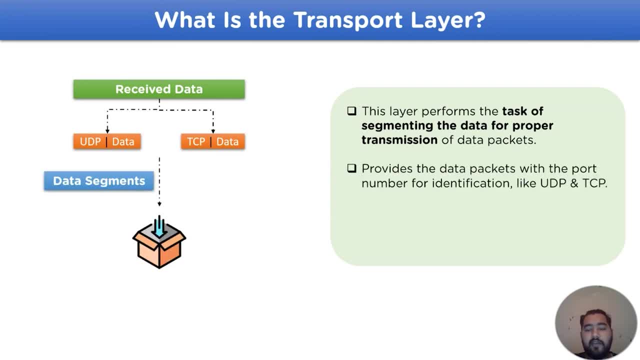 and check there is no error in the data using different network protocols, for example UDP and TCP. Then these data segments are shared over the connection and non-connection network services. It also identifies suitable communication channel for the data. Now let's move on to. 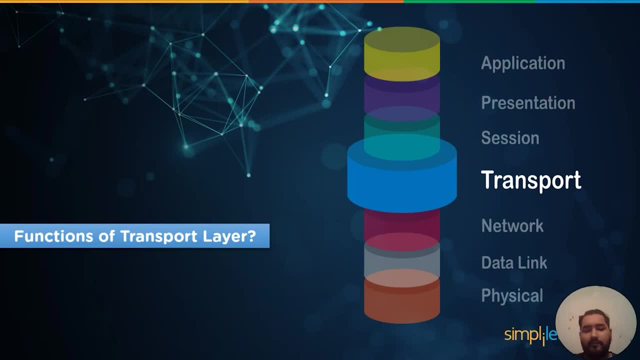 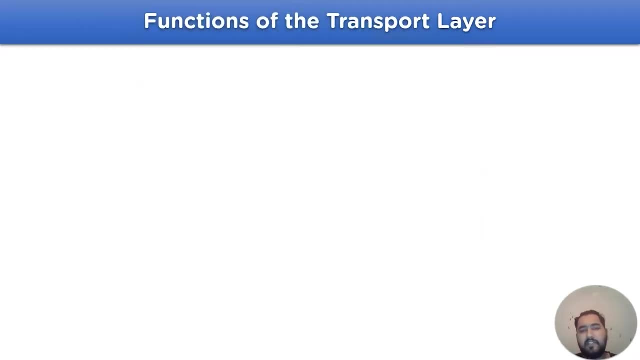 the next heading, that is, the functions of transport layer. Before we begin with the actual functions of the transport layer, let's take a look at the data flow that occurs between the multiple layers of the OSI model and the transport layer. To begin with, the session layer. 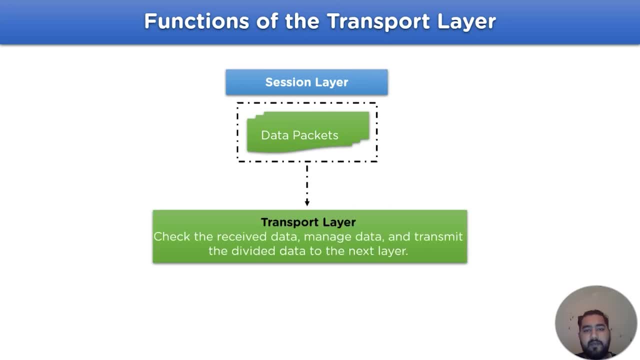 We'll share data packets over to the transport layer, where it will be checked for various errors or corruption in the data received. It is then transmitted into smaller units over to the next layer. In between this, multiple protocols are applied in the transport layer, for example TCP, UDP, a CTP and then these: 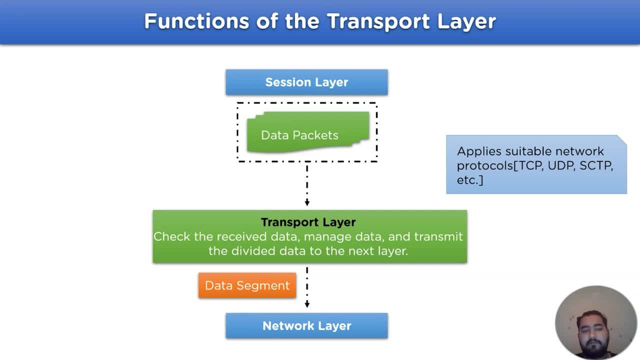 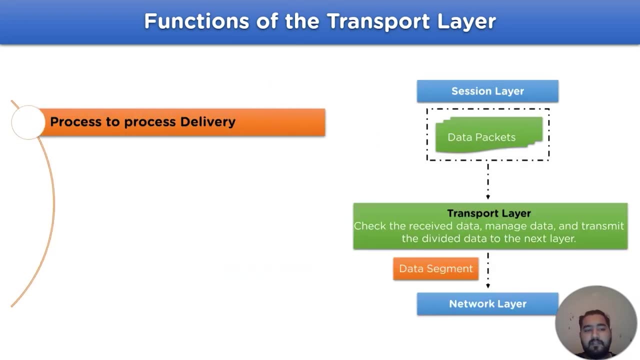 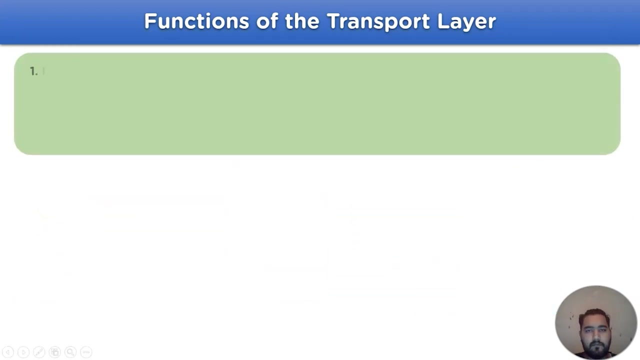 data segments are shared over to the bottom layer. Now let's take a look at the functions available for the transport layer. The first is process to process, delivery, multiplexing and deep multiplexing, congestion control, flow control and, lastly, error control. Let's move on with each of them in detail. 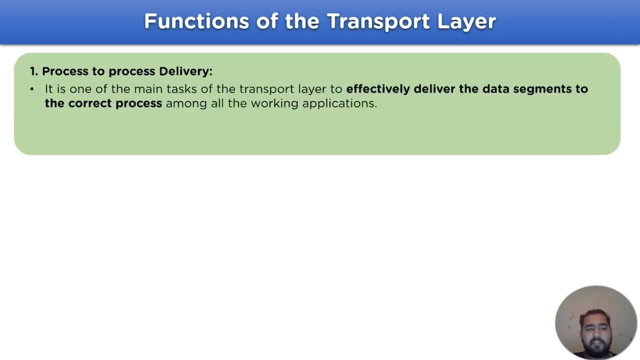 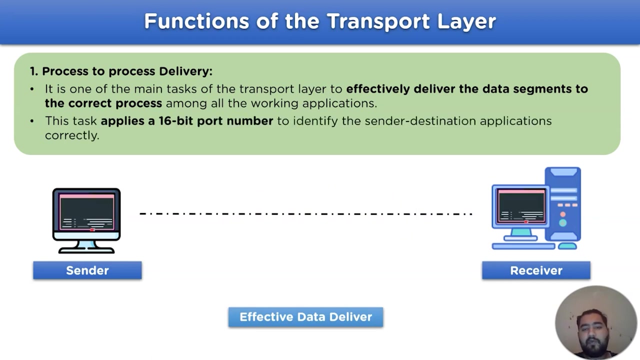 The first is process to process delivery function. In this function it is one of the main tasks of the transport layer. It is designed to effectively deliver data segments to the correct process among all the working application. over the sender side, This task applies a 16 bit port number to identify the sender destination application. 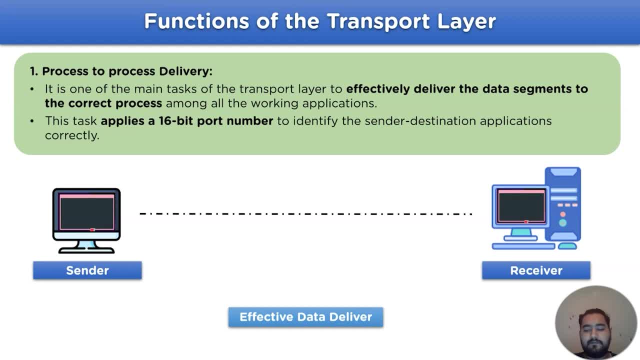 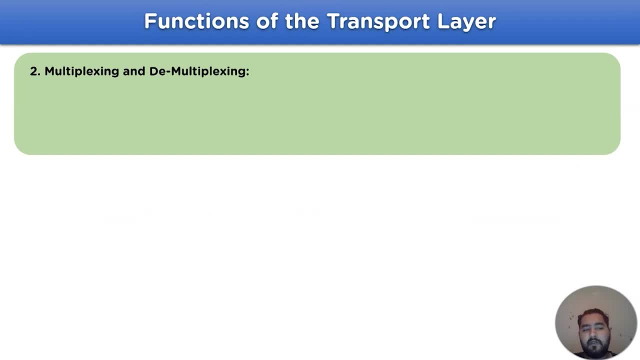 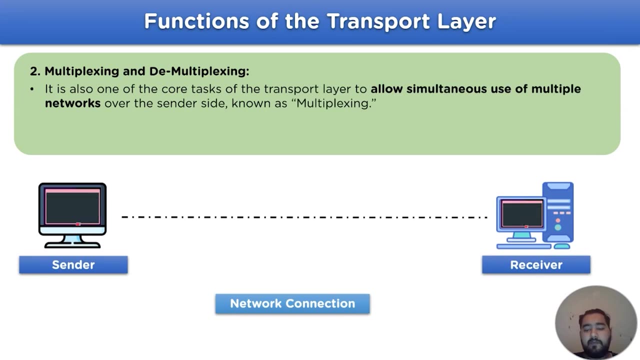 correctly to transmit data over the network channel. Now let's move on to the next function, that is, multiplexing and demultiplexing. The first term is multiplexing. It is also one of the core task of transport layer to allow simultaneous use of multiple networks over the sender side, and this is known as 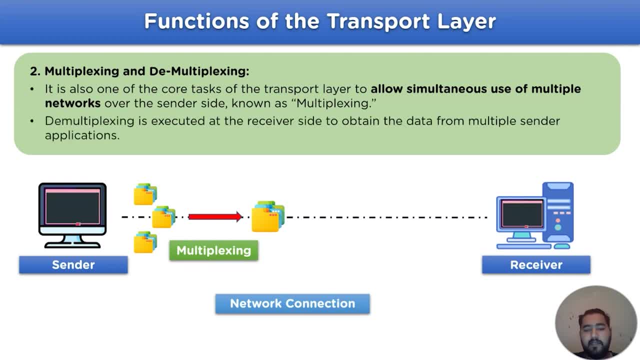 multiplexing, Whereas demultiplexing is executed at the receiver end to obtain data from multiple senders application. Now let's move on to the next function, that is, congestion control. The first term is multiplexing. It is also one of the core tasks of transport layer to allow simultaneous use of multiple 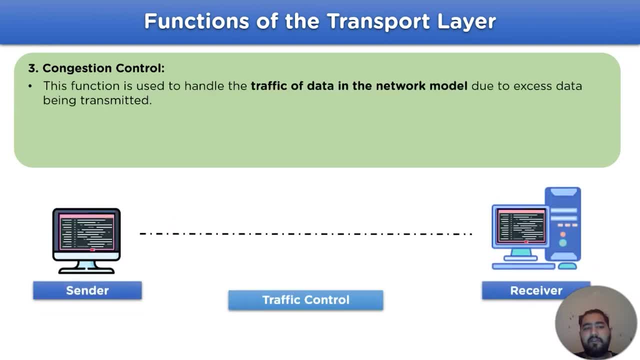 networks over the sender side, and this is known as demultiplexing. This function is used to handle traffic of data in the network model which arises due to access data being transmitted over the network channel. The congestion control of data is handled in two parts. 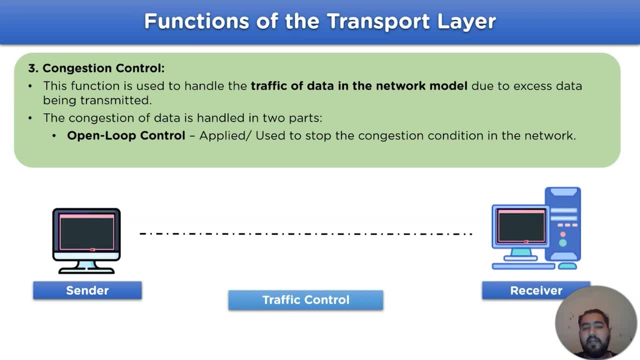 The first is open loop control, which is applied to stop congestion condition in the network channel, Whereas the second control is known as closed loop control. This control is developed along the network network highway and is applied to eradicate congestion situation in the network model. Now let's move on to the next function in the transport layer. 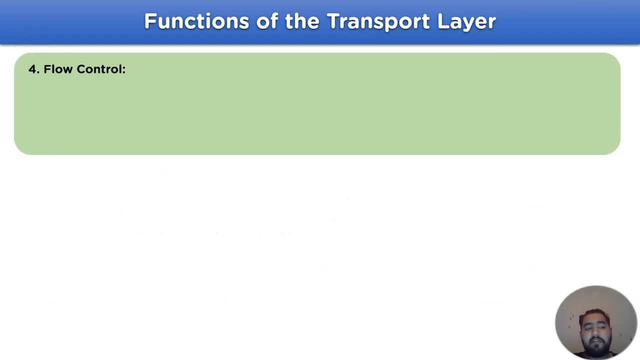 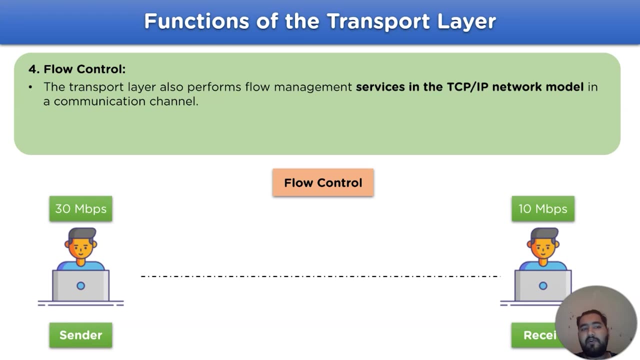 The next function is known as flow control. The transport layer performs flow management services in the TCPIP network model in a communication channel. Después veilChannel, Write a裡 to handle traffic, the network model. To know more about the sliding window protocol principle, you 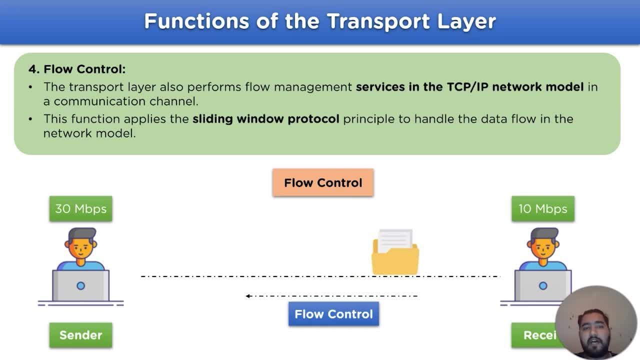 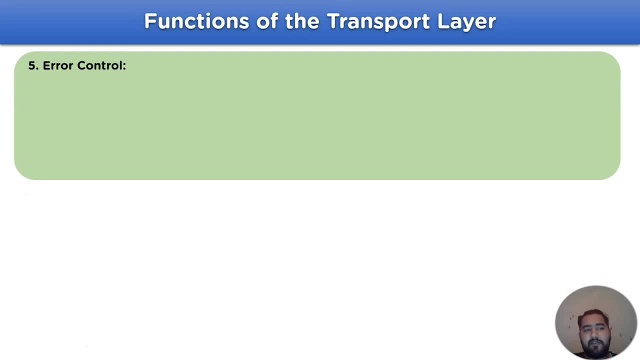 can watch our previous videos. Now let's move on to the last function of the transport layer. The last function of the transport layer is known as error control. The transport layer also checks errors in the information received from the upper layer. in the OSM model, Error detection is performed using the